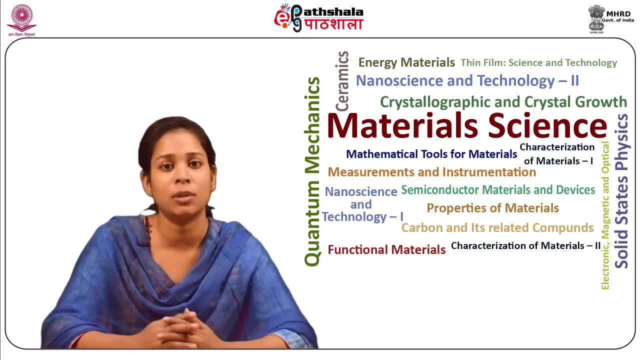 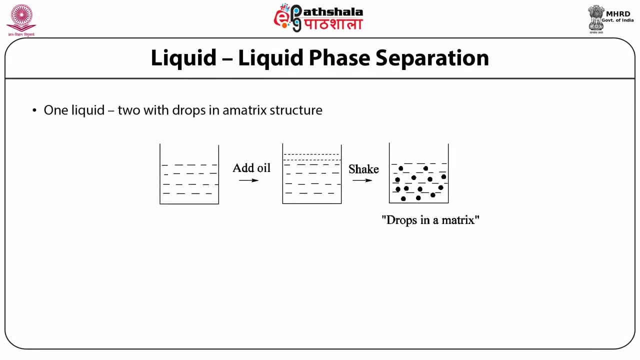 or it can be heterogeneous nucleation. So the processes of nucleation and growth have already been discussed previously, and in the further slides we will be discussing the phenomena of liquid-liquid phase separation. First we will discuss liquid-liquid phase separation. If we take some amount of water in a container and add oil to it, then the two form a separate. 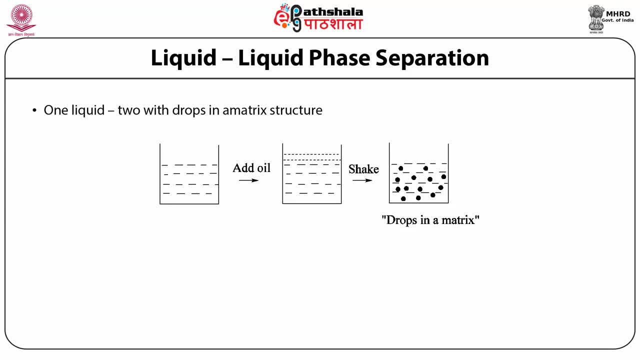 layer and do not mix. That is, the oil and water are immiscible. If the container is closed and shaken vigorously, the oil breaks into droplets which are dismissed in the major phase, that is, the liquid-liquid phase separation. If the container is closed and shaken vigorously, 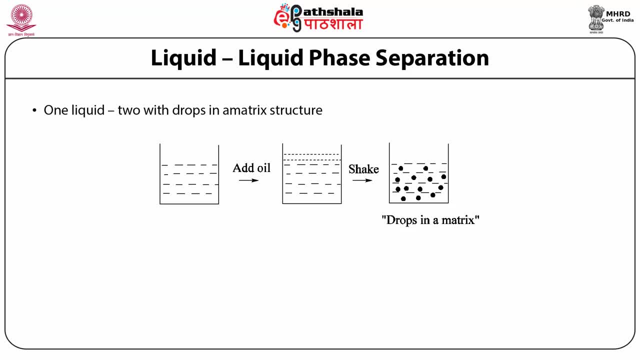 ie water. The two ie, oil and water, are still immiscible, but the morphology has changed from a layer structure to drops dispersed in a matrix structure In glasses. also, a single liquid phase can separate into two immiscible phases under certain conditions. 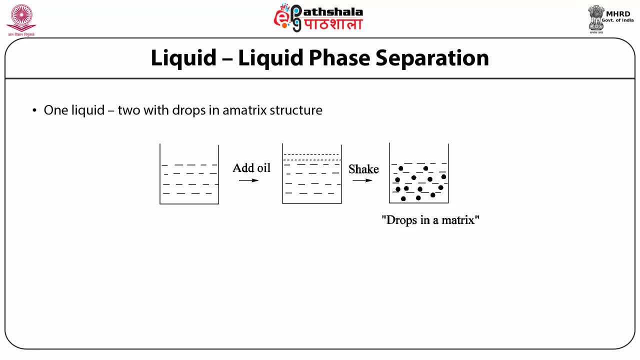 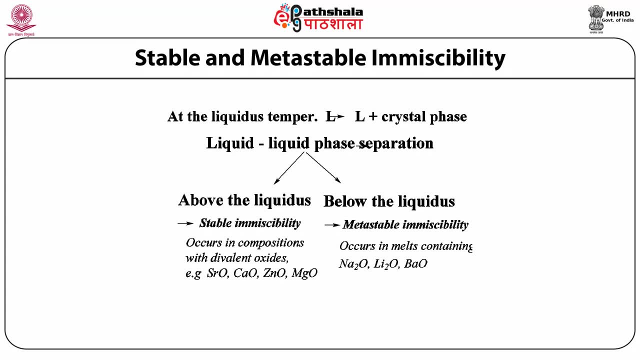 This is called liquid-liquid phase separation. A liquidous temperature is called or defined as the temperature at which a crystalline phase begins to separate out from the liquid. The liquid-liquid phase separation can occur above the liquid or below the liquid. The former is called the stable immiscibility and the latter is called sub-liquidous or 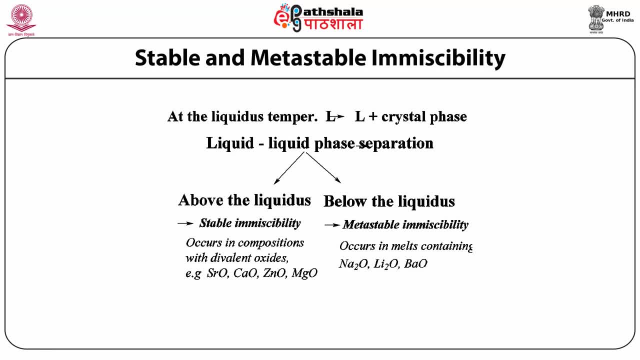 metastable immiscibility. Examples of systems in which stable immiscibility occurs are compositions containing divalent metal oxides, Example- Strontium oxides, Chlorine oxides, Ammonium oxides, Calcium oxides, Iron oxides, Zinc oxides, Magnesium oxides. 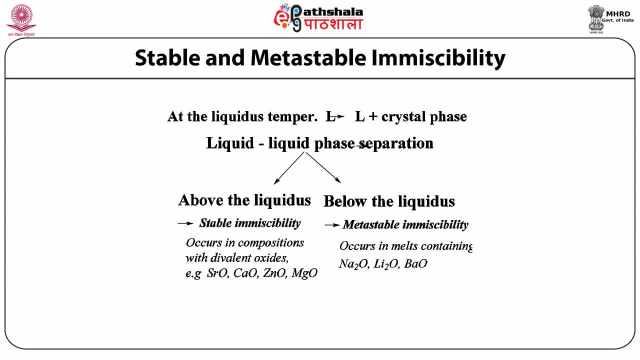 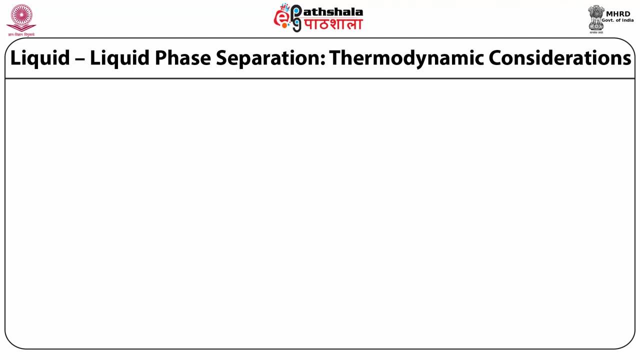 While the sub-liquidous immiscibility is found in silicate mels containing Na2O- ie sodium oxide, Li2O- ie lithium oxide and BaO- ie barium oxide. These systems have an S shape: liquid S. Now let us discuss about the thermodynamic considerations. 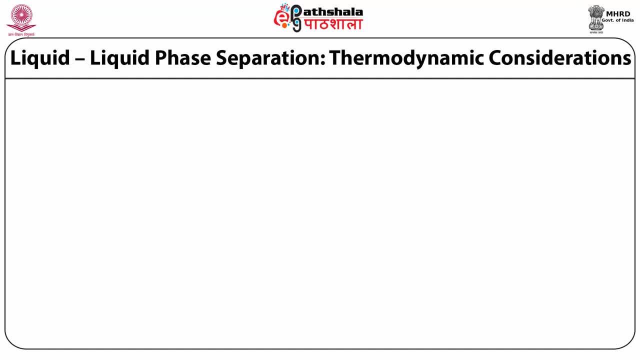 in liquid phase separations. A single phase would separate into two phases if the process leads to a reduction in the free energy. The free energy of mixing of two phases can be written as: delta GM is equal to delta HM minus T, delta SM, where G is the grips free. 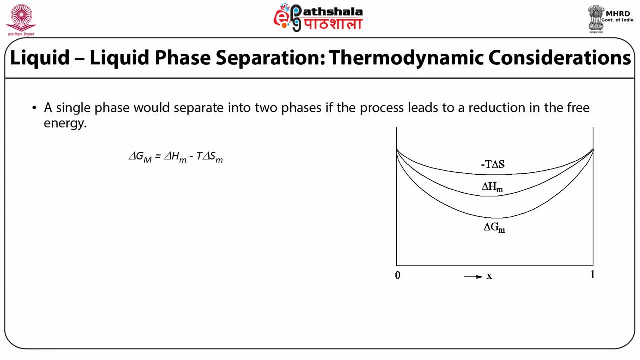 energy, H is the enthalpy and S is the entropy. So, students, you can see on the right hand side the figure showing the free energy versus composition at high temperature, where the system exists as a single phase At a sufficiently high temperature, the second term. 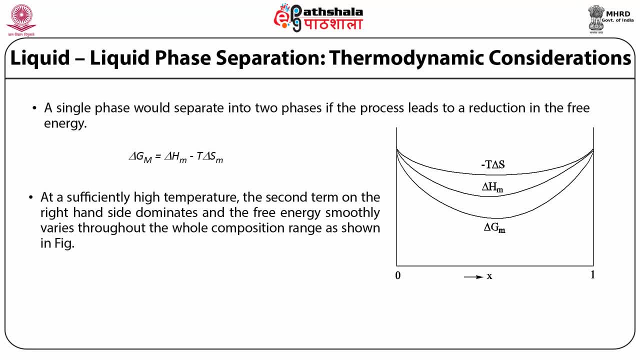 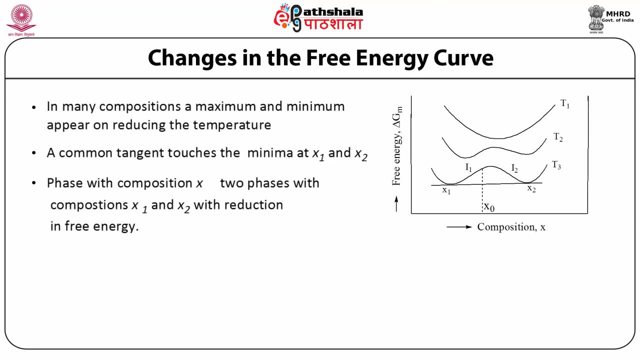 of this equation on the right hand side dominates and the free energy smoothly varies throughout the whole composition range. If the first term is large and positive or if the temperature is reduced, a maximum and two minima occur in the delta G versus composition plot as the temperature is reduced. 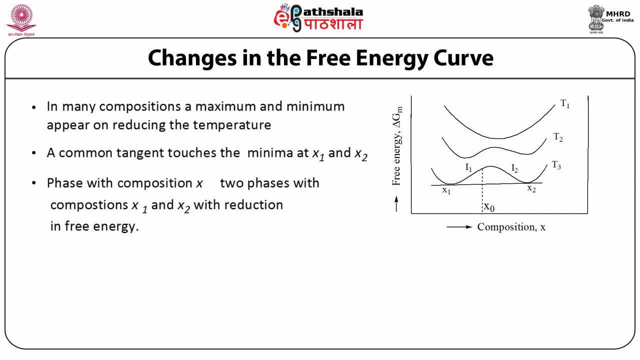 below a certain temperature, called upper critical temperature. This upper critical temperature is also known as consolute temperature, which is shown in the figure Below. this temperature, say, T3 is the free energy and S is the enthalpy. So, students, you can see on the right hand side. 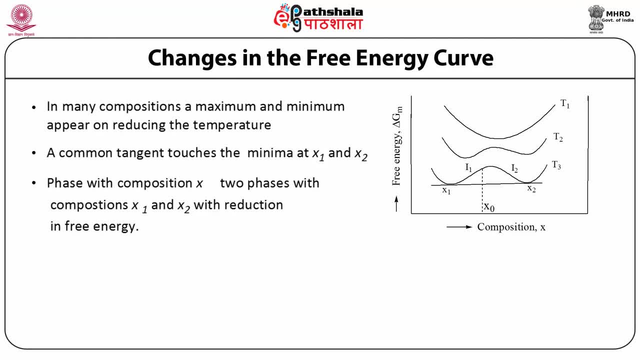 this is the free energy and S is the enthalpy and this is the enthalpy. So, students, you can see on the left hand side T3. so here T3 is consolute temperature or upper critical temperature. So at T3 a common tangent can: 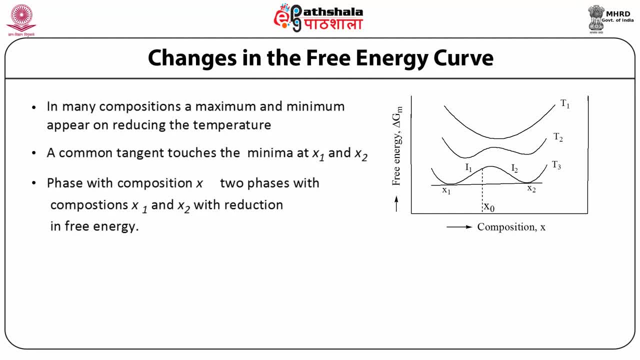 be drawn to the two minimas. The tangent touches the minima at compositions x1 and x2.. Now let's discuss about phase separation by nucleation and growth and by a nuclear solution. Let's discuss about phase separation by nucleation and growth and by a nuclear solution. So in this case, 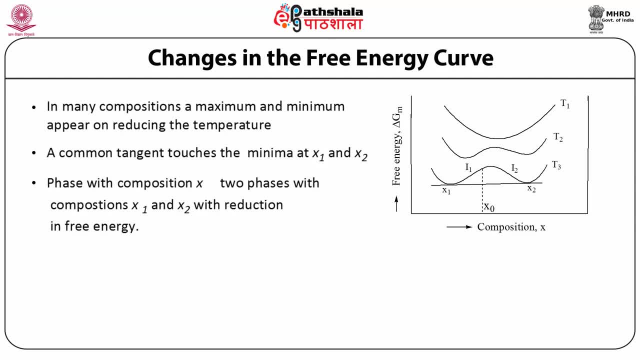 phase separation by nucleation and growth and by a nuclear solution. Now let's discuss about phase spinodal and decomposition. Let the solution have an average composition. Let G0 be the average free energy of an atom and G be the free energy of any one atom in the solution. 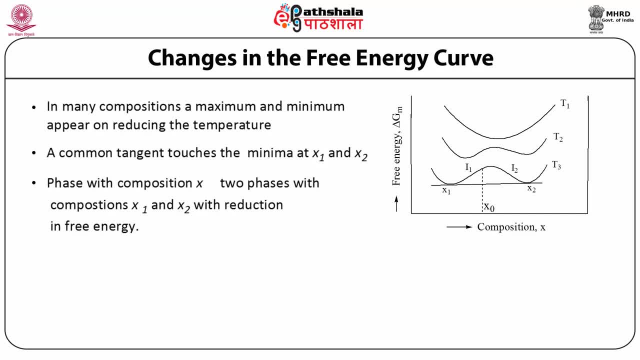 The probability of an atom having the free energy that is G is given by the Boltzmann distribution, which is given as: F of delta G is equal to A times exponential minus delta G by KT, where delta G is equal to G minus G0.. The probability of N atoms having the 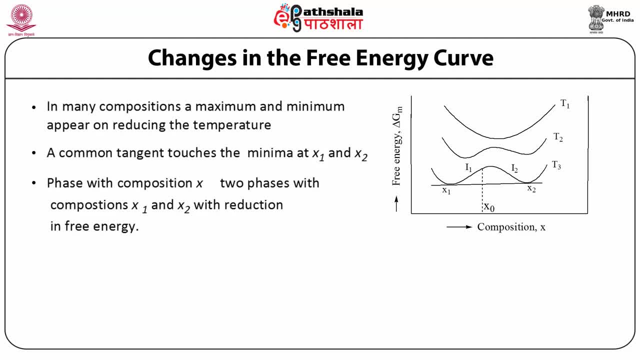 same energy. G simultaneously is F of delta G. F is equal to A times exponential minus N delta G by KT. Assuming the delta G is small and expanding, by Taylor series one gets: G is equal to G0 plus 1 by 2 d square G by dx. 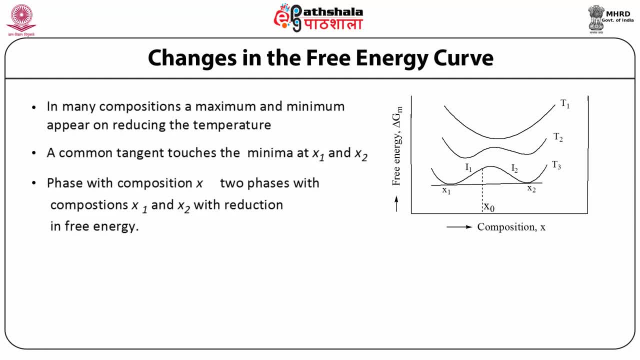 square times, x minus x0 square and so on, Neglecting higher order terms. as the composition fluctuations x minus x0 is very small. Now, substituting G minus G0 is equal to delta G, we get the probability of a small fluctuation. 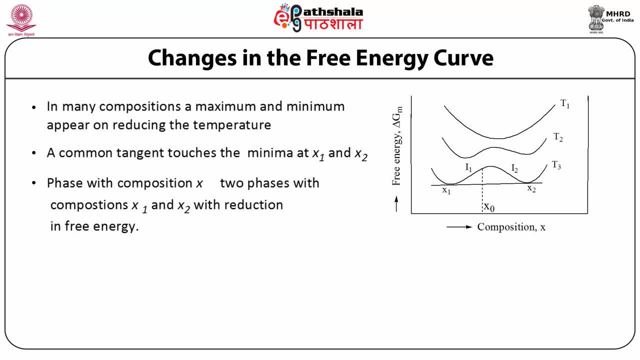 involving N atoms, which is given as: F is equal to A times exponential minus delta G by delta G by KT. F is equal to A times exponential minus N delta G by dx square, and so on, Neglecting larger order terms, as the composition fluctuations x minus x0 is very small. 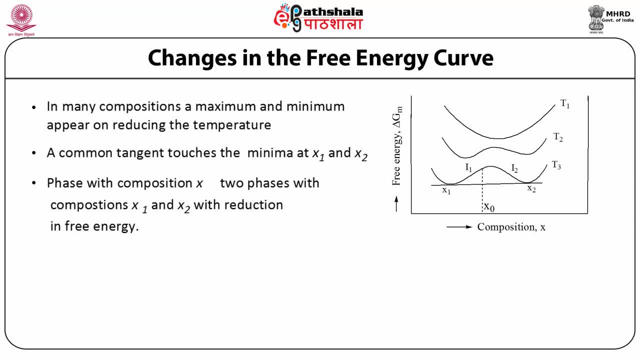 But F is equal to A times exponential minus N into x, minus x0 whole square into d square G by dx square complete divided by 2 KT. From this equation it is seen that the probability of the fluctuation will be large if the curvature of the free energy curve d square G by dx. 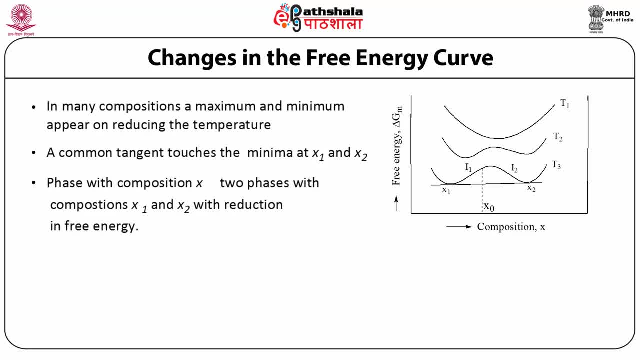 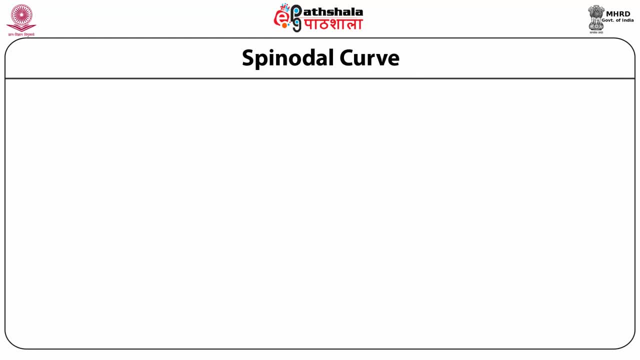 square is negative. So in this case the fluctuations will occur simultaneously and spontaneously. Now let us come back to the previous figure, in which the composition versus free energy at different temperatures is drawn. The tangent to the 2 minima touches the minima. 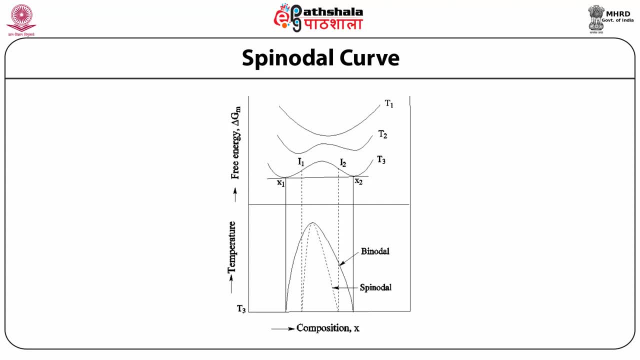 points x1 and x2.. Points I1 and I2 are the inflection points at which the quantity d2, x by dx squared, the curvature of the curve is 0.. For compositions between the inflection points, the curvature is negative. However, the curvature is positive. 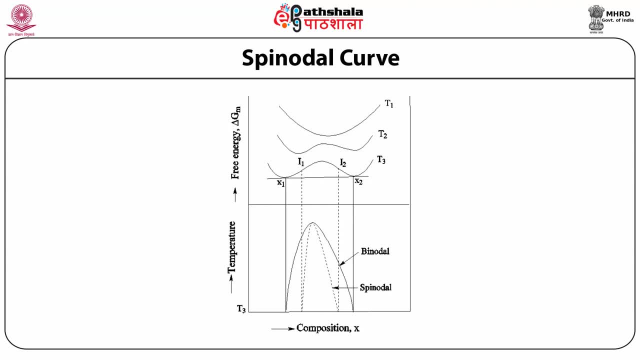 outside the composition range between I1 and I2.. In the lower diagram one can see that the locus of the points of the tangency at different temperatures are drawn. This curve has a dome-like appearance and is called binodal curve. Also drawn is the locus of the points. 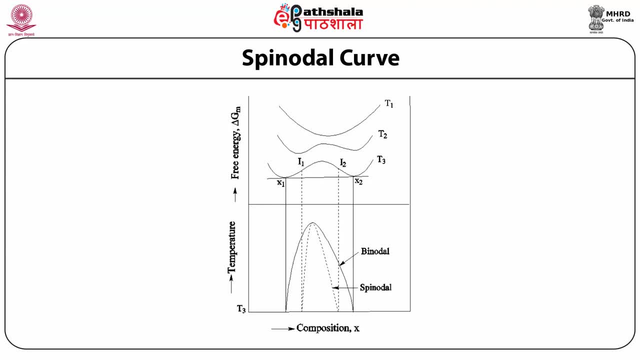 I1 and I2 at different temperatures, shown as a dotted curve Within the binodal dome. this curve is called spinodal curve. In the composition range included by the spinodal curve the curvature is negative. So any small composition or fluctuation. 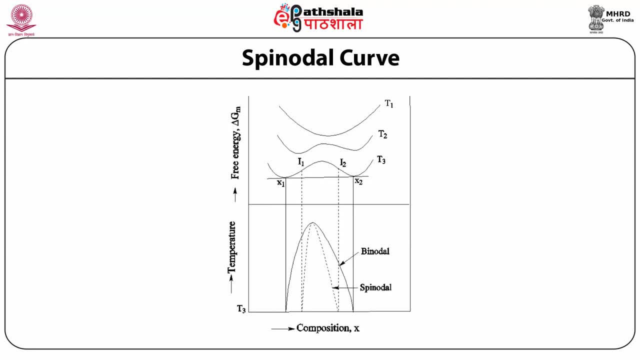 in a solution of this overpass over all composition would be accomplished by a decrease in the free energy, and so it would be stable. The system can easily phase separate into two compositions differing by a small amount in composition. The system is therefore stable with respect to phase separation. 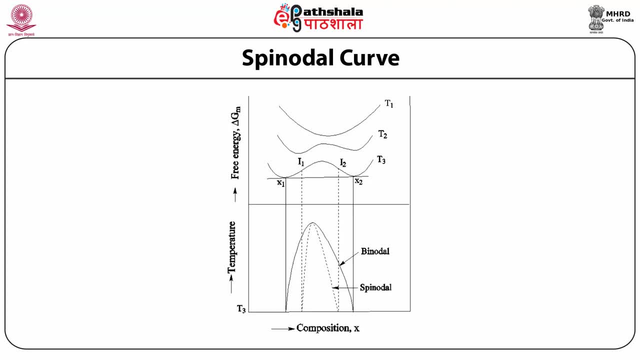 So in this case any local fluctuation in the composition would grow. The composition of the two phases would change until they attain the composition given by the common tangent ie, x1 and x2.. This process of formation of two phases is called spinodal decomposition. 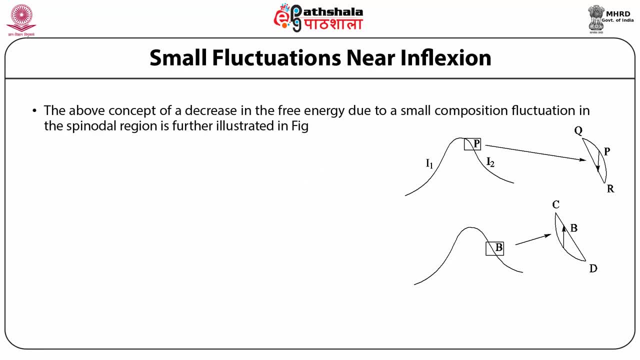 The above concept of a decrease in the free energy due to a small composition fluctuation in the spinodal region is further illustrated in this figure. For an initial composition P, small fluctuation leads to compositions Q and R. The free energy change follows the arrow and decreases. 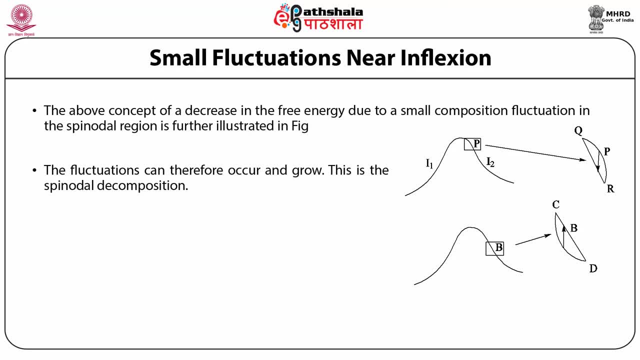 The fluctuations can therefore occur and grow. This is the spinodal decomposition. For any composition between the spinodal dome and the binodal dome, the situation is as shown in the figure. In this case, a smaller fluctuation leads to an increase in free energy. 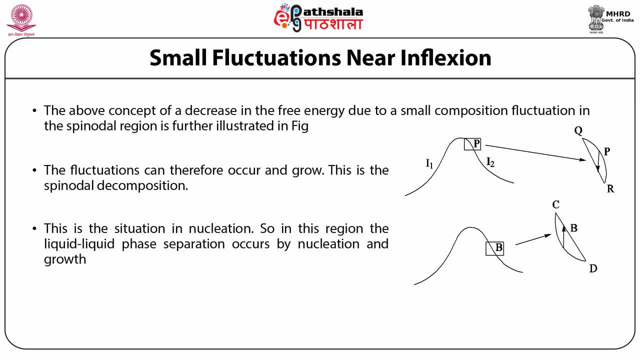 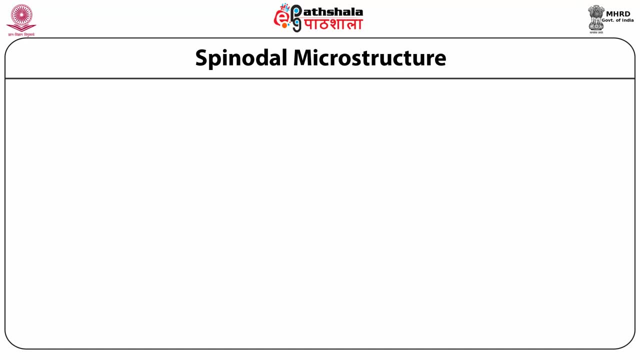 This is the situation in nucleation. So in this case the liquid-liquid phase separation occurs by nucleation and growth. Now let us discuss the spinodal decomposition. The morphology produced in the two cases is quite different, ie spinodal and binodal. 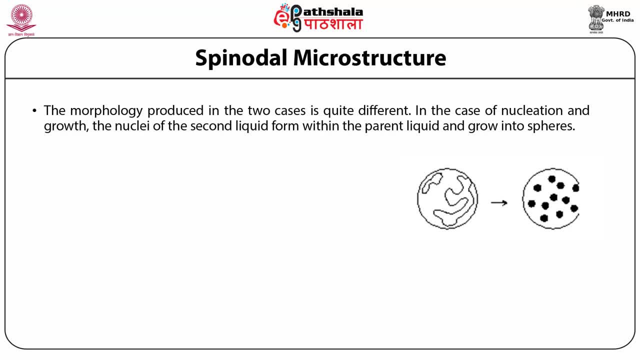 In the case of nucleation and growth, the nuclei of the second liquid form within the parent region, within the parent region in the parent liquid, and grow into spheres. The morphology in this case is called spheres in a matrix microstructure. This can be seen in this figure. 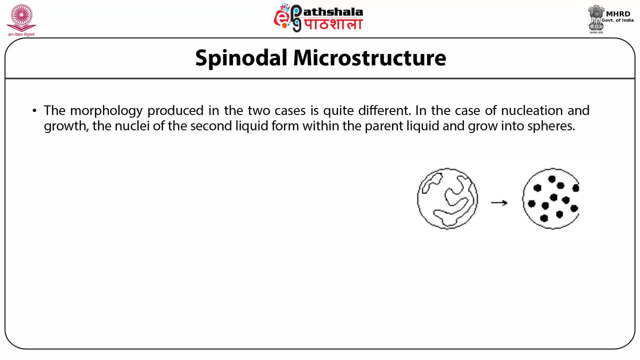 So in the spinodal decomposition a phase with initially uniform composition separates into two phases which initially differ only slightly in composition. But with time the composition fluctuation sharpens and eventually an initially bicontinuous structure transforms to a droplet structure. However, in case of spinodal decomposition, the morphology is: 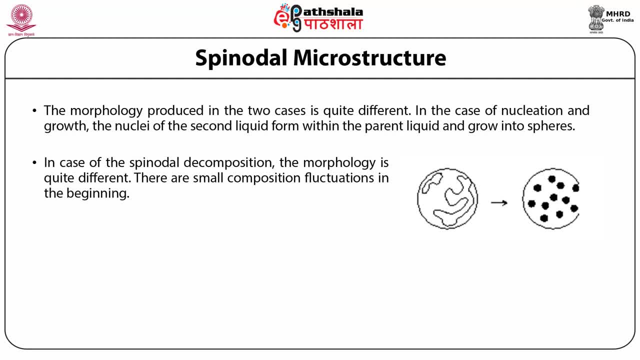 quite different. There are smaller composition fluctuations in the beginning, which we have discussed. The boundaries between two phases are diffused and the two phases are interconnected and spread throughout the whole volume. Both phases will have high degree of connectivity, The interfaces sharpen with time and eventually a morphology similar to that of nucleation. 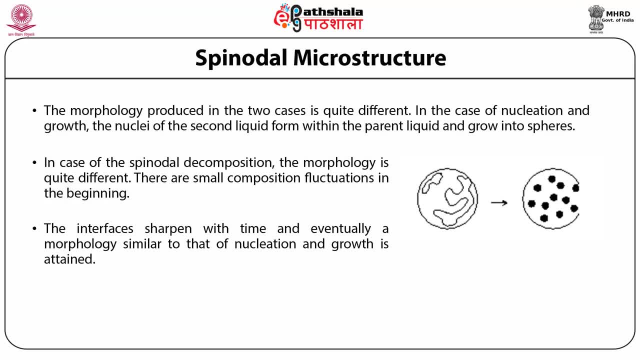 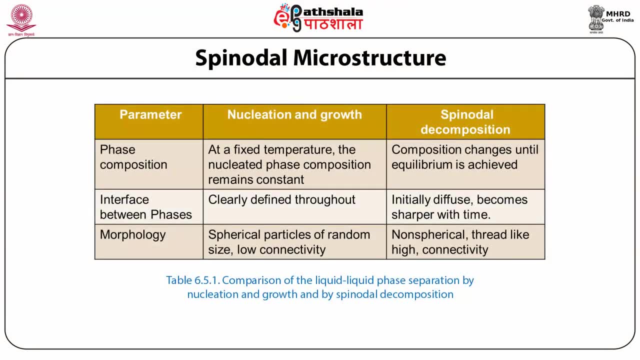 and growth is attained. These two morphologies are explained earlier. Now this table summarizes the differences between phase separations, nucleation and growth, and by spinodal decomposition. So you can see that the parameter, that is, phase composition, differs in both the cases. First case is nucleation and growth and second is 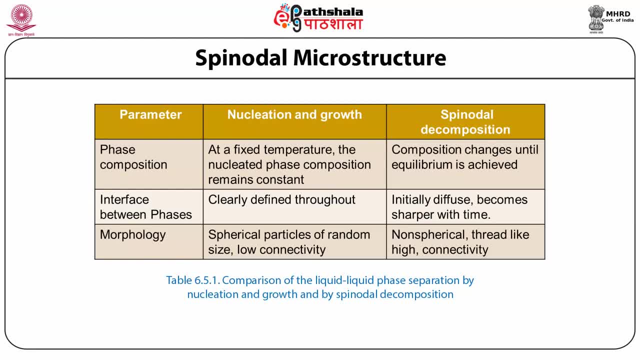 spinodal decomposition, So at a fixed temperature the morphology is different. The morphology in phase separations depends upon thevideo station zitten. The nucleated phase composition remains constant, whereas in case of spinodal decomposition the composition changes until the equilibrium is achieved. 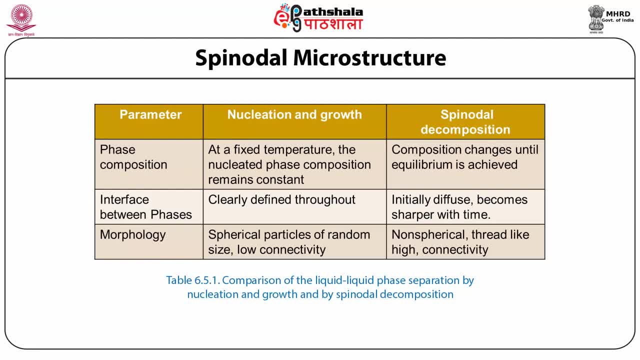 However, if we discuss about interface between phases, these are clearly defined throughout. whereasin case of spinodal decomposition, they are initially diffused and then become sharpens with time time. The third is morphology: In case of nucleation and growth, morphology of spherical. 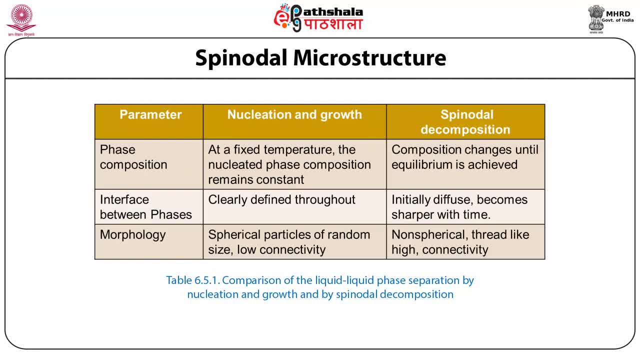 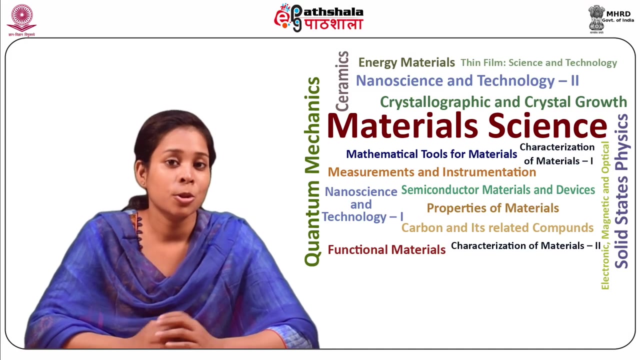 particles are of random size, with low connectivity, Whereas in case of spinodal decomposition, the non-spherical morphology is observed, which are thread-like, and they have high connectivity. So, students, let's now summarize what we have learned in this module. So, students, we have learned that a liquid phase mils can undergo phase changes in several ways. 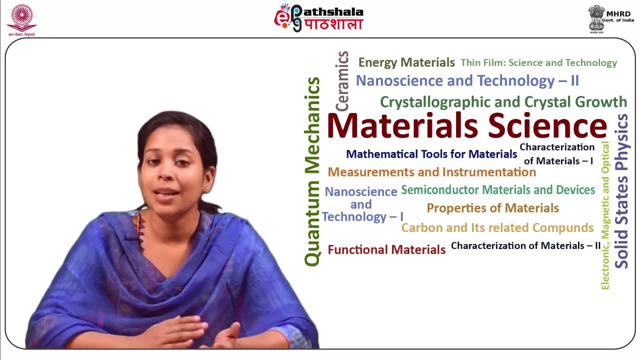 and these are. it can be using liquid-liquid phase separation by homogeneous nucleation and growth. Second, it can be liquid-liquid phase separation by spinodal composition. Third, crystallization by homogeneous or heterogeneous nucleation. Next is modification into rigid glass and subsequent crystallization to glass ceramic. 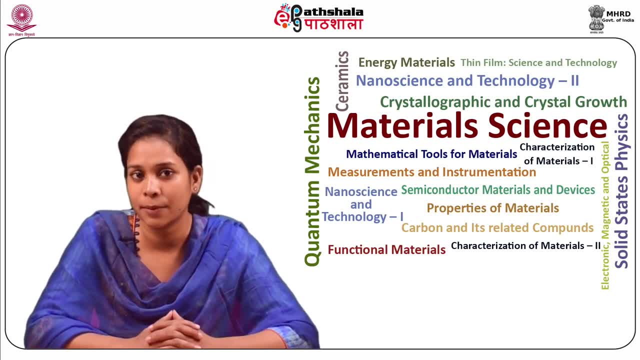 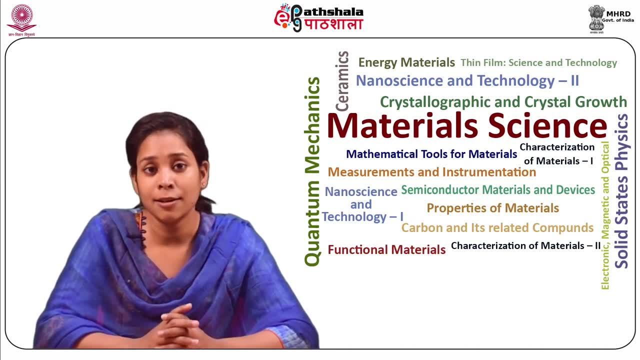 by an appropriate heat treatment. Moreover, we have learned that liquid-liquid phase separation can occur if two minima and a maxima appear in the free energy versus composition plot. as the glass melt is cooled, this can happen above the liquids temperature, in which case it is called stable immiscibility. 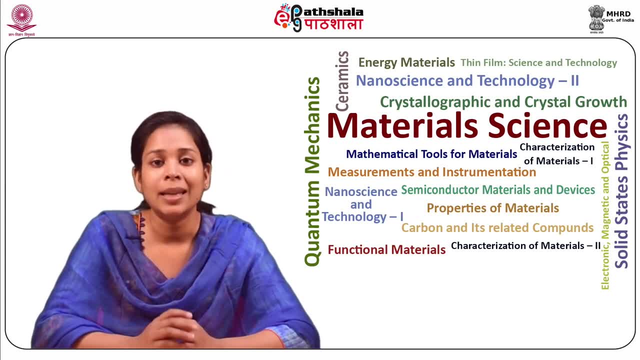 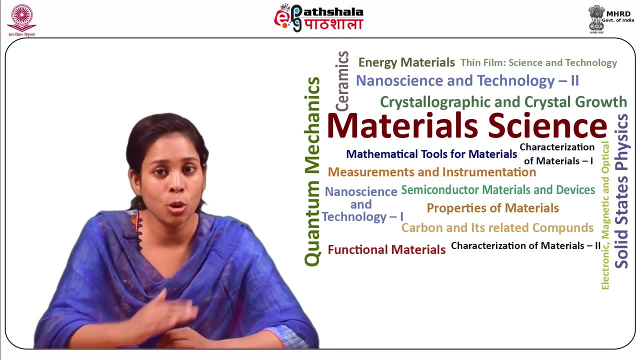 or below the liquidus temperature. in the later case it is called metastable immiscibility and the locus of the minima in the free energy versus composition plot at different temperature leads a dome shaped curve called binodal curve. so the locus of the infliction points in the free. 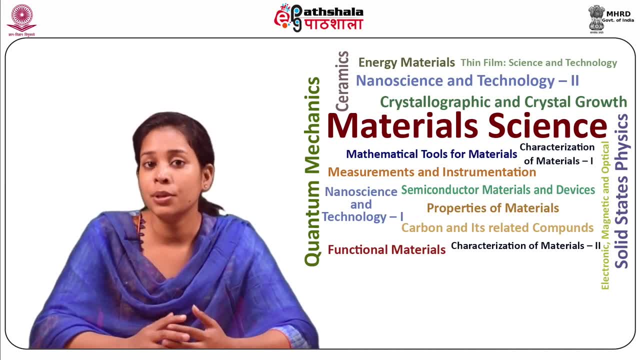 energy versus composition plot produces another curve within the binodal curve, and this curve is called spinodal curve. so for compositions between binodal curve and spinodal curve the phase separation occurs by nucleation and growth. for compositions within the spinodal curve, the free energy reduces, even if